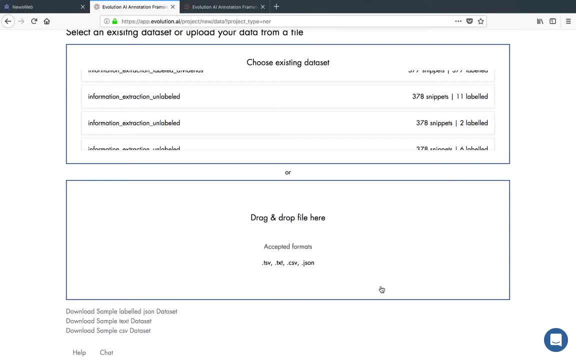 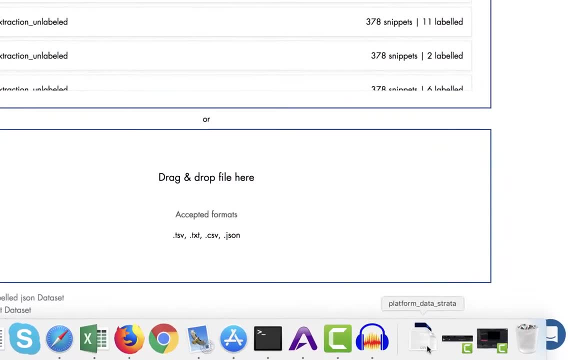 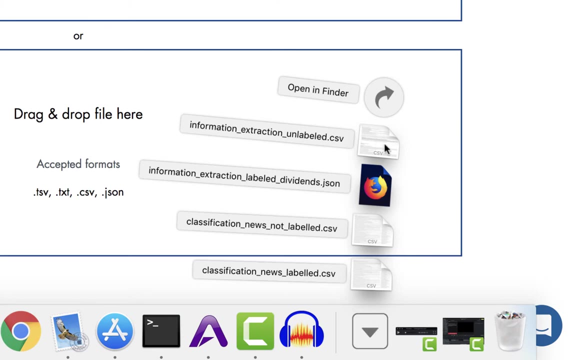 a file into the drag-and-drop section. For this demonstration I took over 300 dividend examples from the Oslo Stock Exchange news web we saw earlier and created a CSV file. The CSV file is called information extraction, unlabeled, and I'll select and drag this into the load file area. So 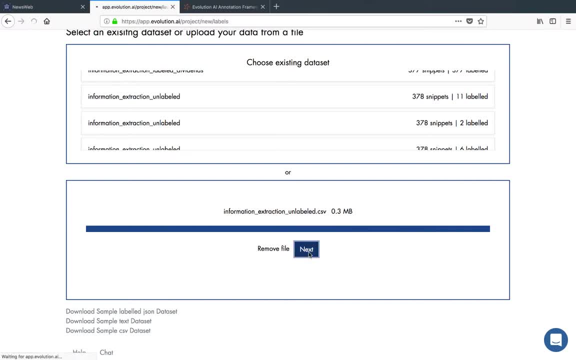 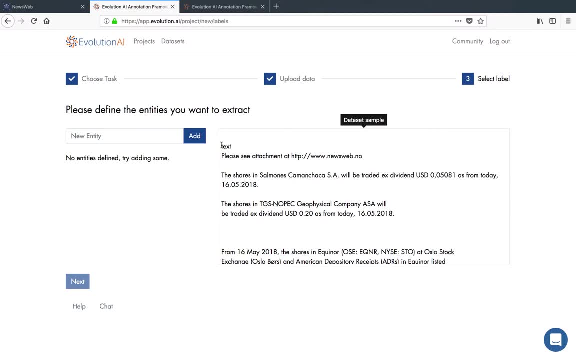 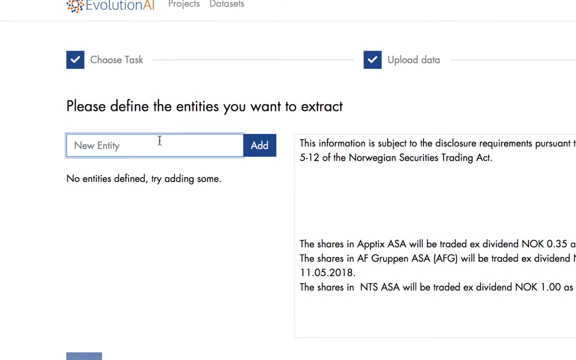 the training data is now loaded into the platform, So I'll select next, and we are ready to add our labels. On the right hand side of the screen, a sample of the uploaded data set is shown. So let's create our three labels. Firstly, I'll create the currency label, then the amount and finally the date label. 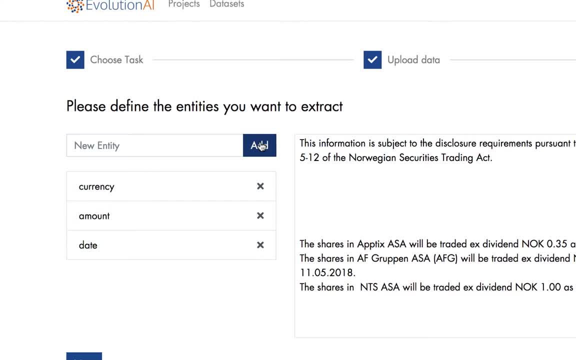 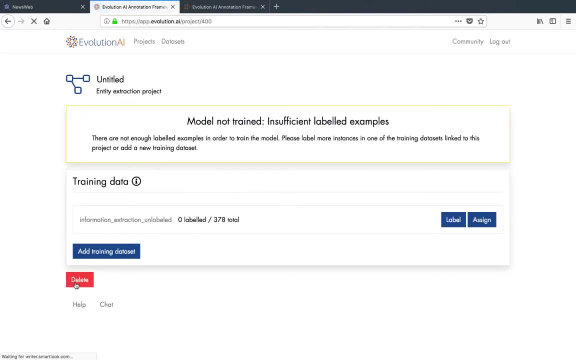 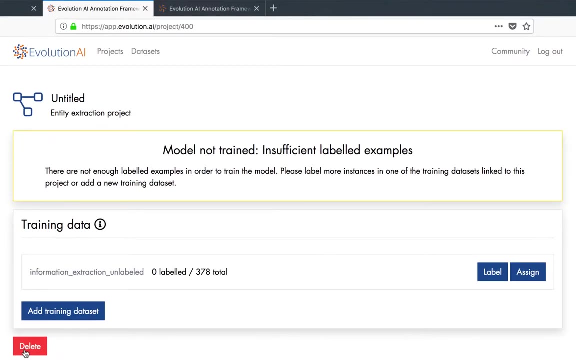 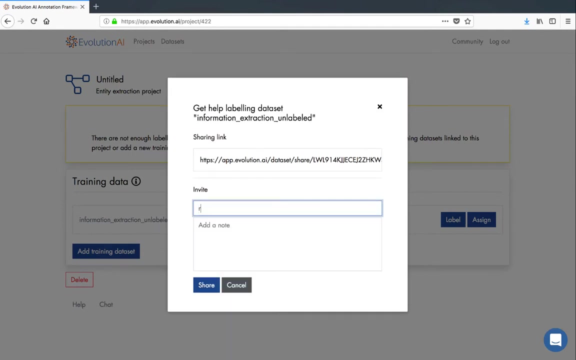 Once I've created the labels, I'll click next And the first thing you'll see is that the model tries to train. In this case, as I haven't labeled any examples, the model can't train. You can use the assign feature to send someone a data set to label. Simply add their email address and a. 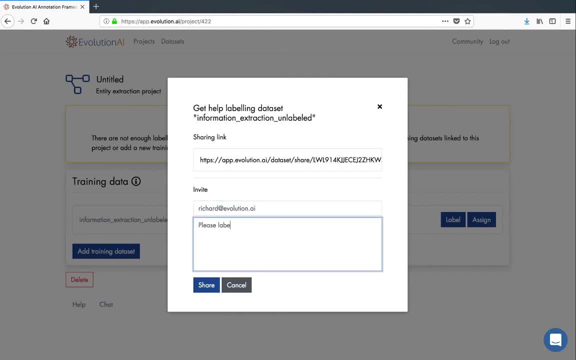 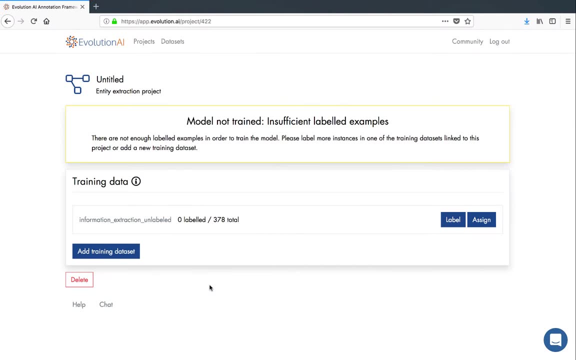 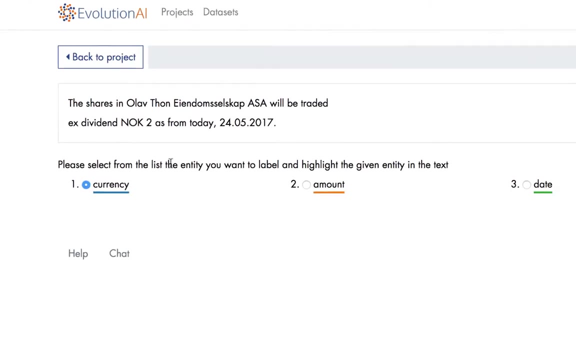 message and they will receive a link to the data set ready to label. So let's label some data, Select label And then we're in the labeling screen. You can see the first of our samples And I'm labeling the currency. Now the amount. 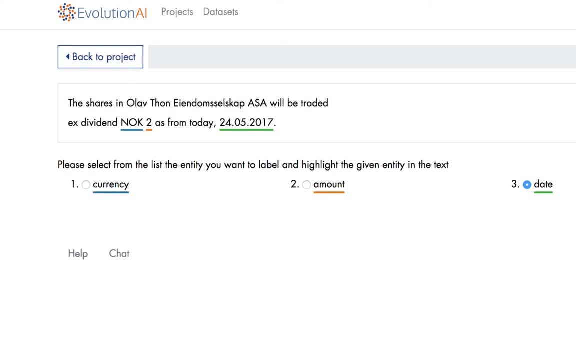 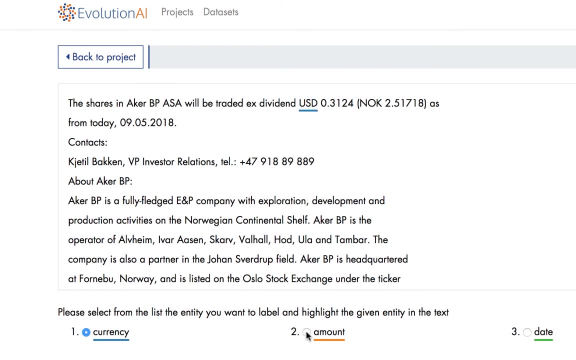 And now the date of the sample. I then click submit. Here's the second sample. Once again I label the currency- US Dollars, the amount and the date. I have multiple currencies in this example, So once again I label the Norwegian Krona, the amount, and I submit. 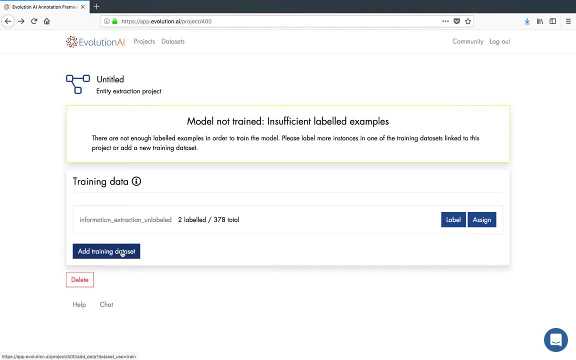 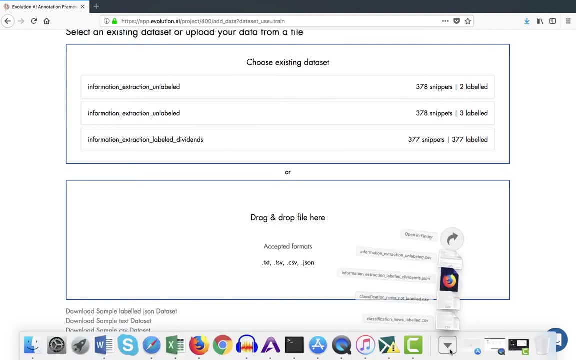 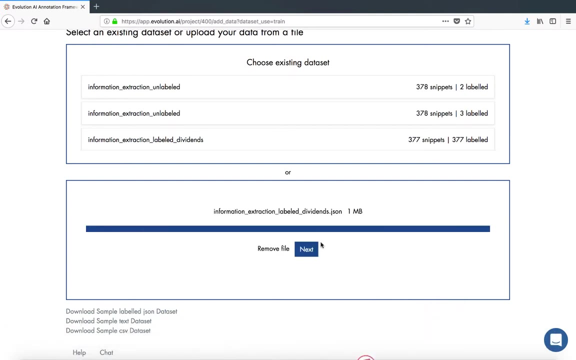 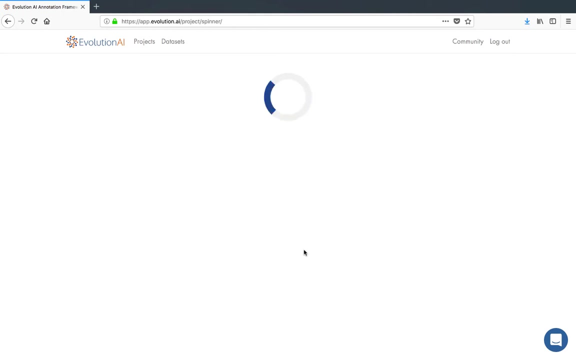 For this demonstration, I created a label training data set called information extraction labeled, And I'll upload this into the platform. like before, The model will now begin training And during this period, the system will give you progress indications. The model will now begin training And during this period, the system will give you progress indications. 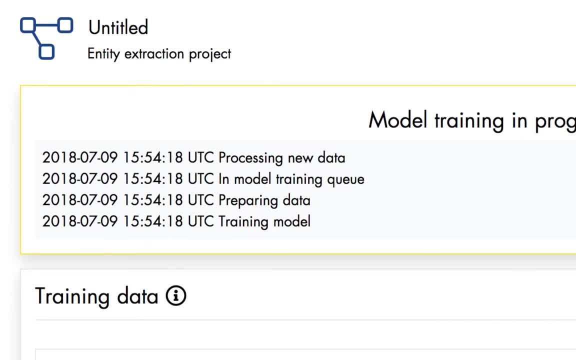 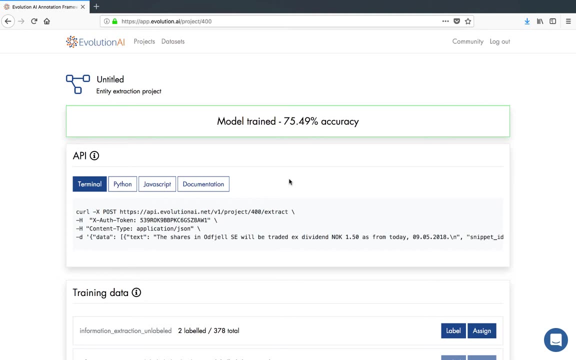 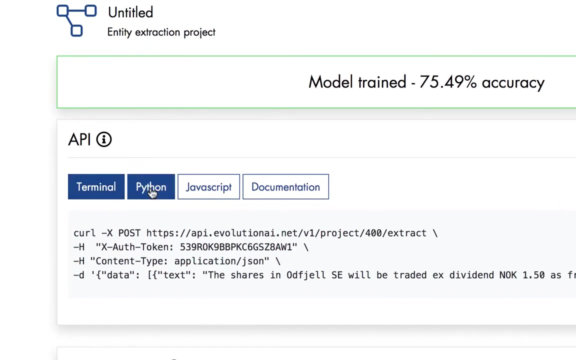 This model will take four minutes to process, So, for the sake of the demonstration, I'll move forward to the train model. So the model has finished training and the platform has generated a REST API which can easily be embedded in your application. The API is generated in either terminal, Python or JavaScript. 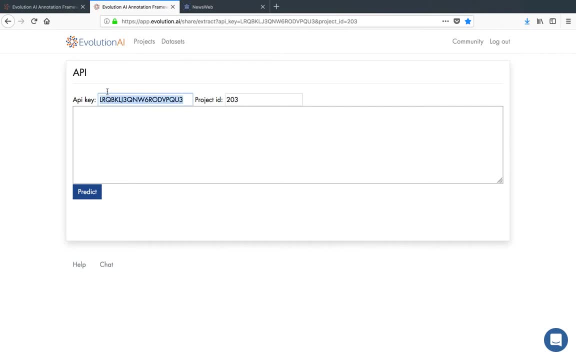 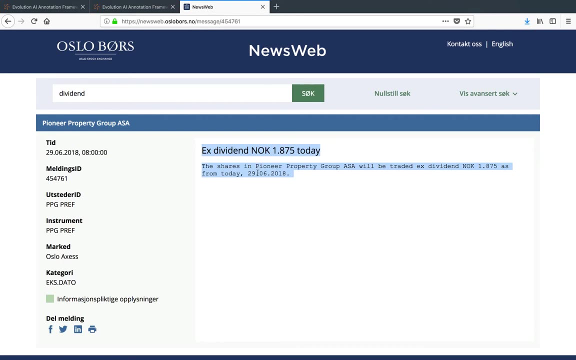 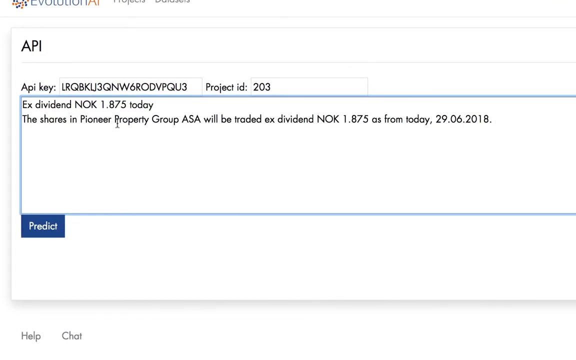 I've created a web application. This calls the API and allows me to demonstrate the model in action. Here's the example from the Oslo News Web. I'm going to cut and paste this dividend report into the web application. You can see, this particular report has two instances of currency and amount and one instance of date. 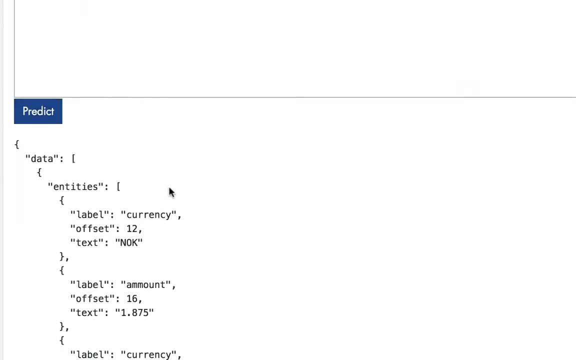 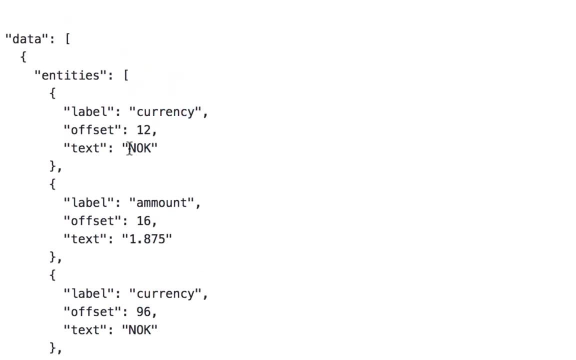 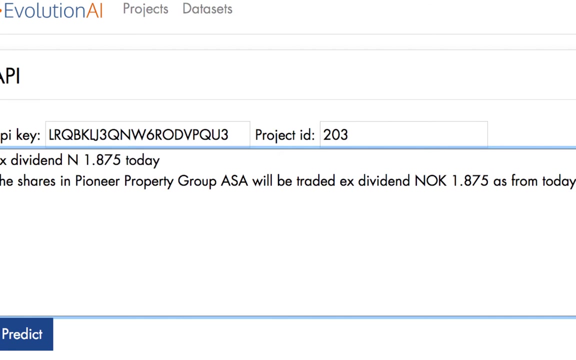 Selecting predict sends the text to the model and the model instantly returns the prediction. You can see the model has correctly predicted the currency as NOK or Norwegian Krona, So let's change the text from NOK to Norwegian Krona and see how the model behaves. 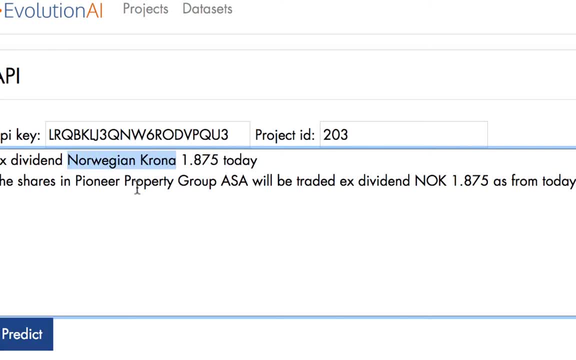 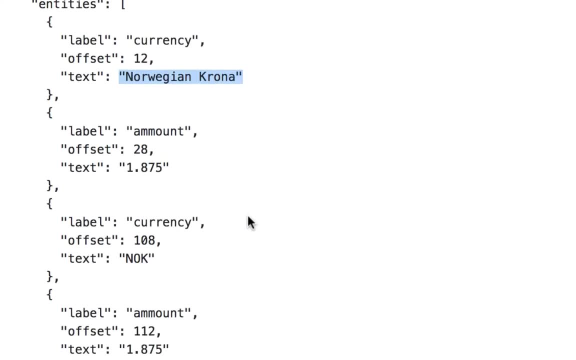 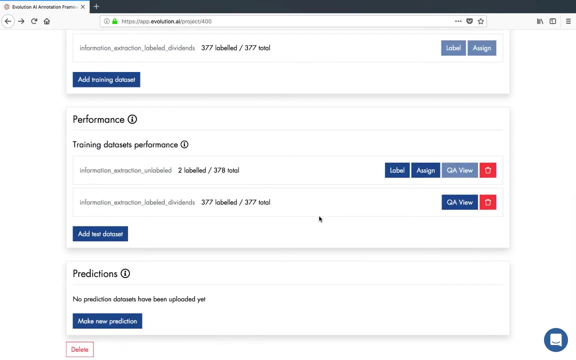 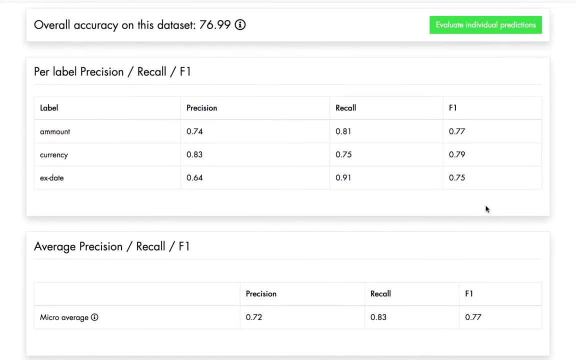 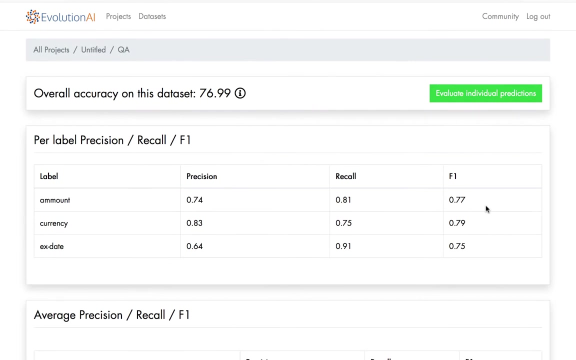 Once again, I select predict and you can see that the model has correctly predicted the currency as Norwegian Krona. Once you've created your model, you can use the platform's QA view to assess the performance. Precision, recall and F1 scores are provided on a per-label and a micro-average basis. 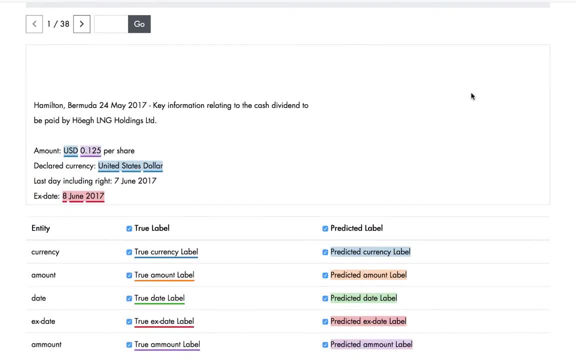 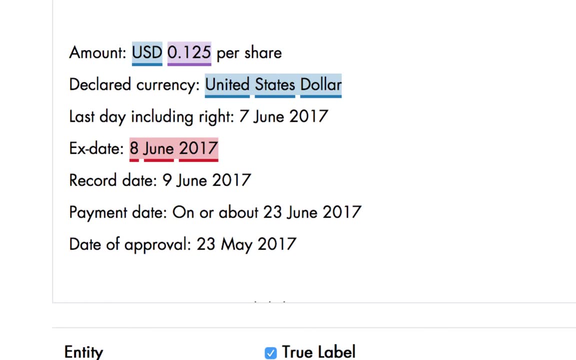 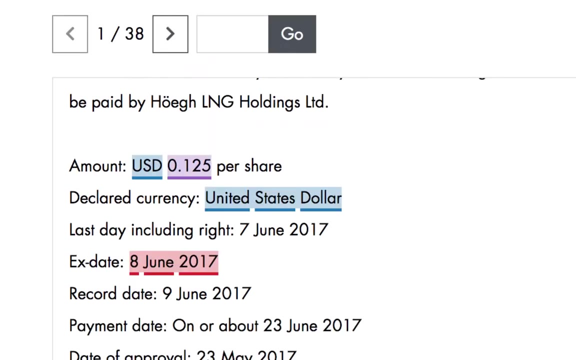 I can also evaluate the individual predictions of the model. The color under the line is the true label and the color that surrounds the text is the actual prediction of the model. If the colors match, the prediction is correct. if they don't match, the prediction is incorrect.